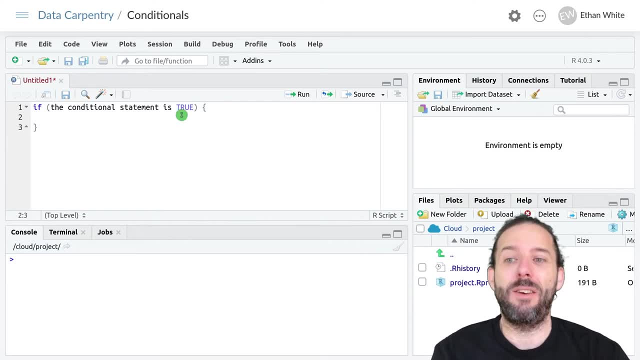 And so this will be the block of code that's executed if the conditional statement is true, And then we'll do something in here. We'll have one or more lines of code that will only get executed if the conditional statement in parentheses is true. 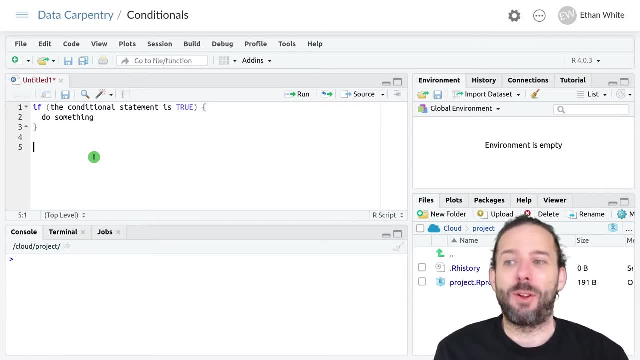 So let's look at an example of what that would actually look like. We'll just start with a value of x that we'll use for checking our conditional statement again. So let's say x is equal to 6. And then we'll have our conditional statement. 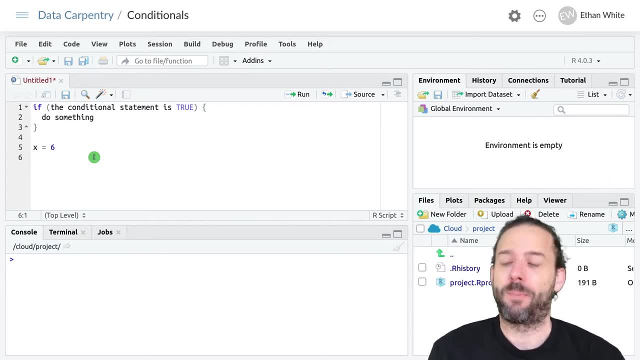 And so let's check to see if x is greater than 5.. And so we'll say, if parentheses, x is greater than 5.. Curly brackets. And then if x is greater than 5, let's square x. So we'll say x is equal to x squared. 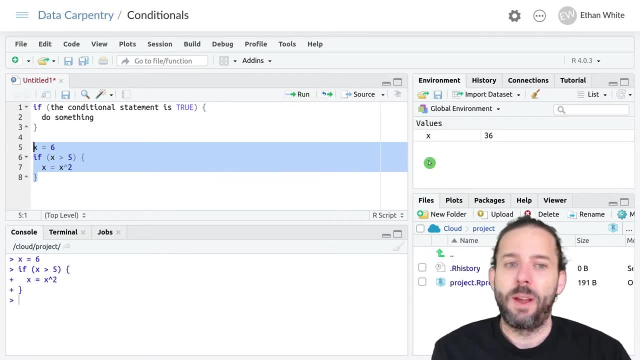 And so if we run this code And then we look and see what x is, We'll see that it's 36.. And so the code x is equal to 36.. Executed like this, We set x is equal to 6.. 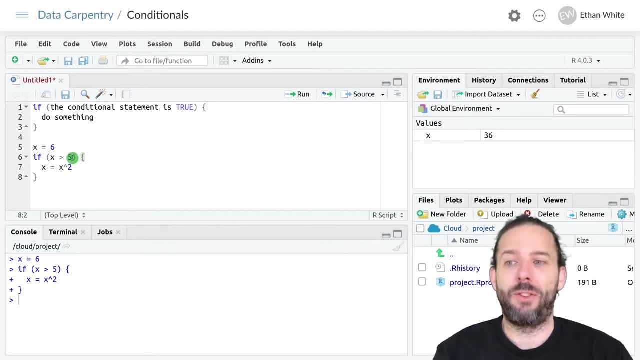 We then check to see if x was greater than 5. It is, So this conditional statement evaluates to true And therefore we run the code inside this block. So we take the value of x, which is 6. Square it And store it back into x. 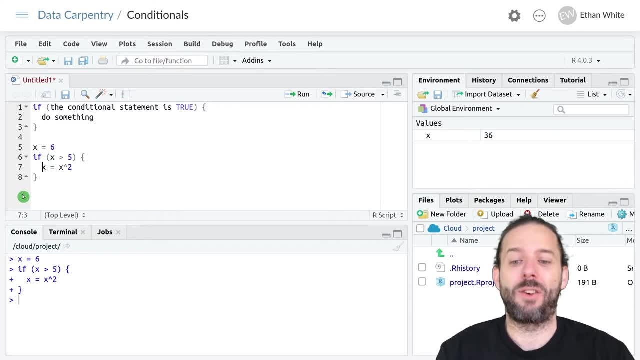 And so that makes x 36.. And then we end our code block. So now let's see what happens if we change x to 4.. Now, if we run this same block of code, What we'll see is that x is equal to 4 over here. 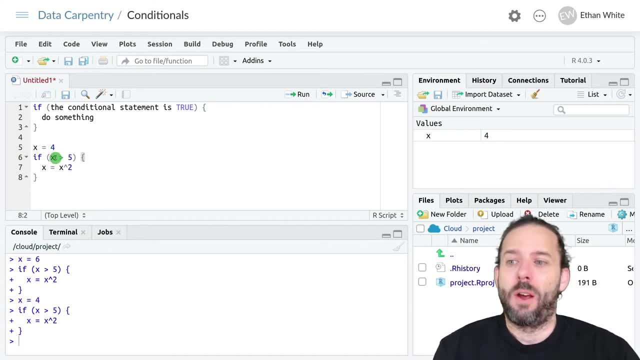 And that's because we set x equal to 4.. We then check to see if x was greater than 5.. 4 is not greater than 5. So this evaluates to false, And so this block of code doesn't get run. 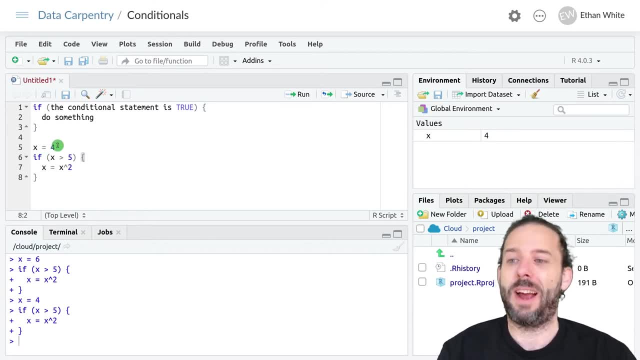 It gets skipped over and doesn't get executed, And so x stays where it was to start with. It's important to keep in mind that this if statement is not a function, So we're using curly brackets to talk about the block of code that's in the if statement. 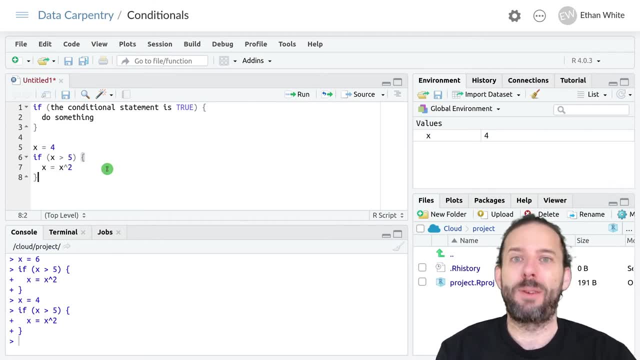 But this is actually out in the broader program. It's not been placed in a function, And so everything that happens here is reflected in our global environment, And that's the basic idea. But let's look at a slightly more real world application of something like this. 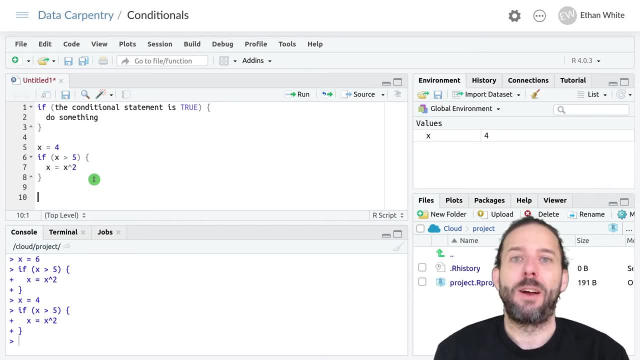 Let's say that we are estimating the mass or biomass of a plant Based on the volume that we've measured in the field. We've done this just with a single equation But, more realistically, the way in which we calculate that mass depends on the specific plant type that we're looking at. 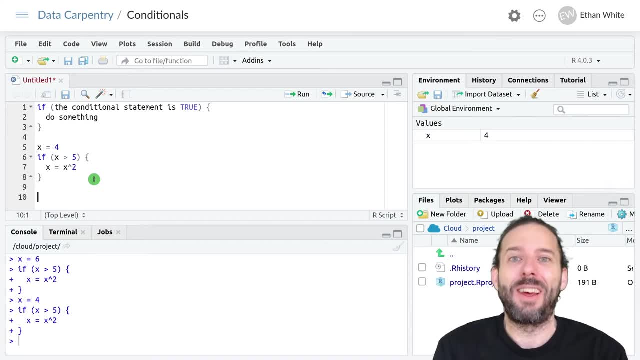 So we wouldn't use the same equation for grasses as we would for trees, for example, And so we can control this kind of behavior then using an if statement, And so we could say: set our veg type, So let's set veg type. 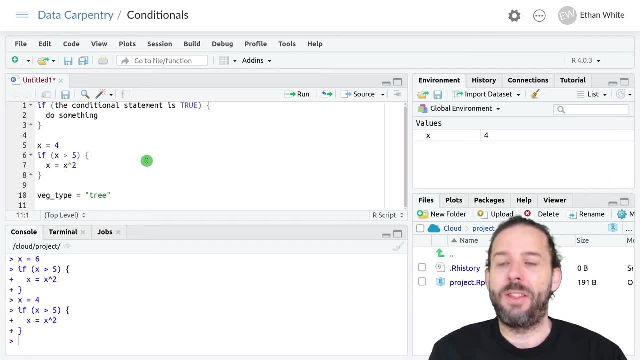 Is equal to tree, And then we could have our volume. And so let's set our volume to 16.08.. And then we could use a conditional to only calculate a mass if the vegetation type was tree. And so we could say, if parentheses- veg type. 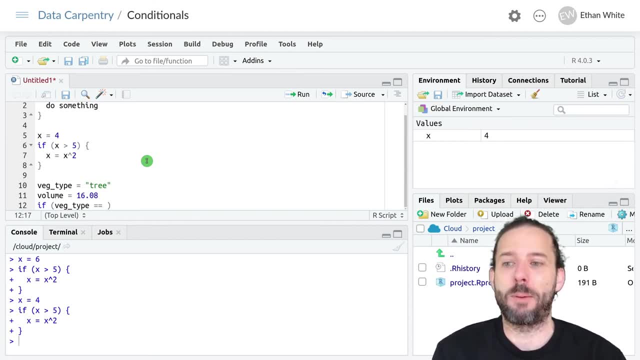 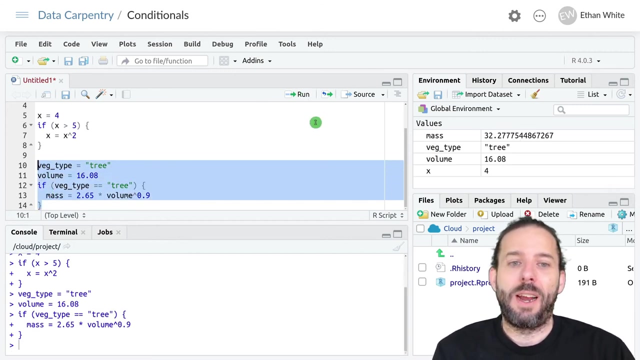 Is equal to Two equals signs- remember For equal to Tree, And then our curly brackets, And then we could say: mass Is equal to 2.65 times the volume raised to the 0.9.. And if we run this code,